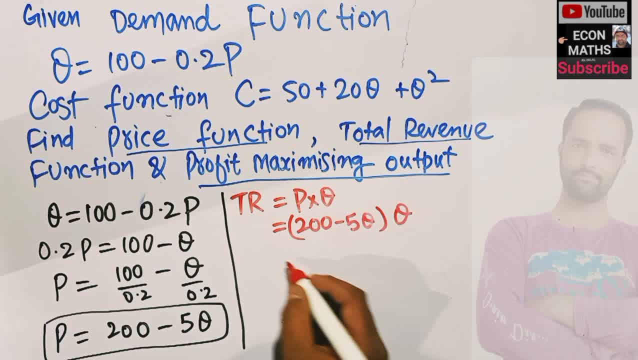 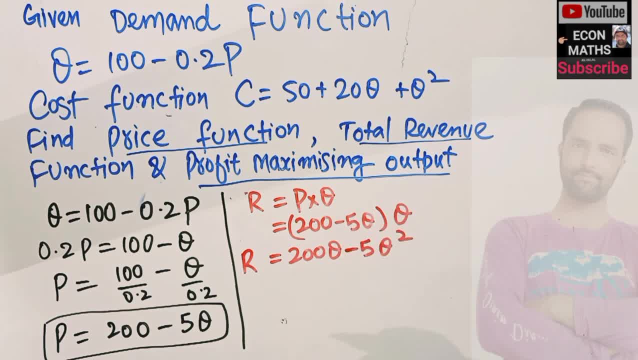 where what we need to find out is the profit maximizing output. So we know that profit is simply equal to total revenue minus total cost. Revenue function is this: So we can write 200Q minus 5Q squared To this, we subtract the total cost function and that is being given us is this: 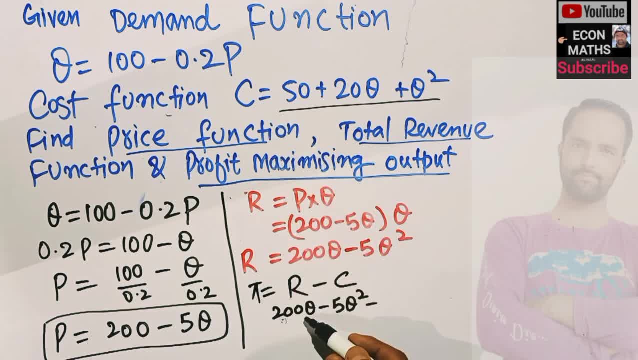 So subtracting this cost function from revenue function will give us the you know profit function. So we have minus 50 minus 20Q, minus Q squared, So this is 200 minus 20.. So we have here 200 minus 20.. So it is simply 180Q. 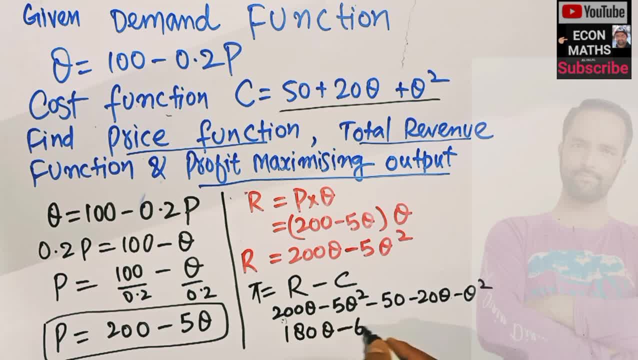 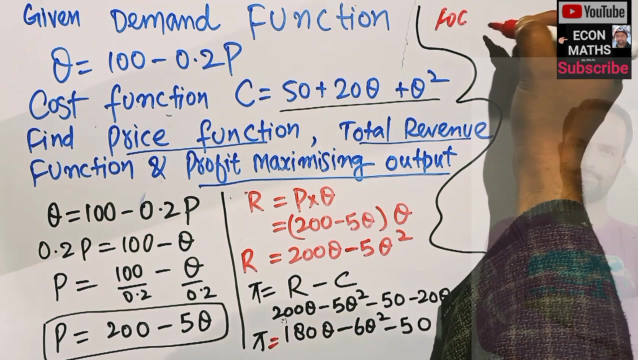 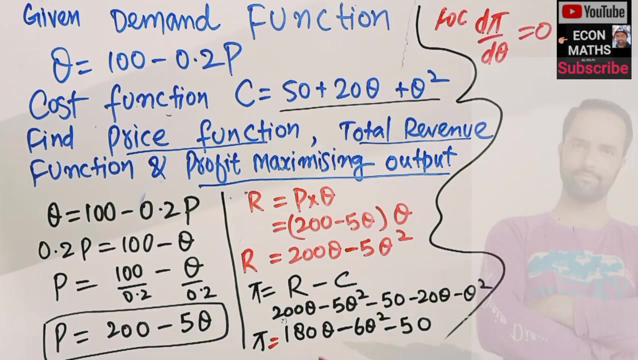 minus 5Q squared. minus Q squared is minus 6Q squared, Then we have minus 50.. This is our profit function. Okay Now, first order condition for profit maximization requires that our marginal profit should be equal to zero. That means d pi upon dQ should be equal to zero, Meaning 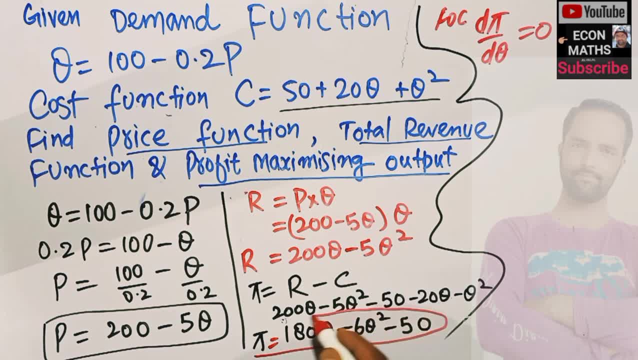 we need to find out the derivative of this profit function with respect to output. Okay, So let me see if I have the space here. Okay, So let us write it here. So d pi upon dQ is equal to zero. 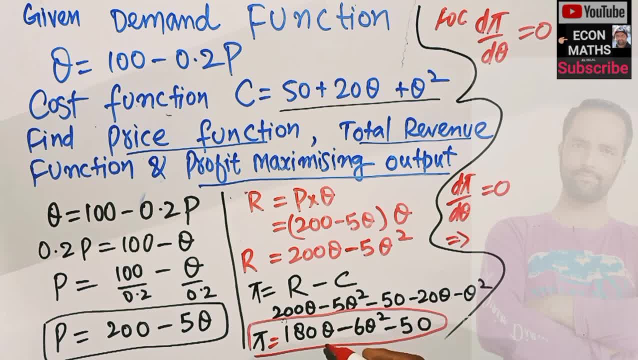 implies taking derivative of this function with respect to Q. Derivative of Q is 1.. So we are left with 180 minus derivative of Q. squared is 2Q. So 2,, 6,, 7, 12Q, 12Q minus derivative of a. 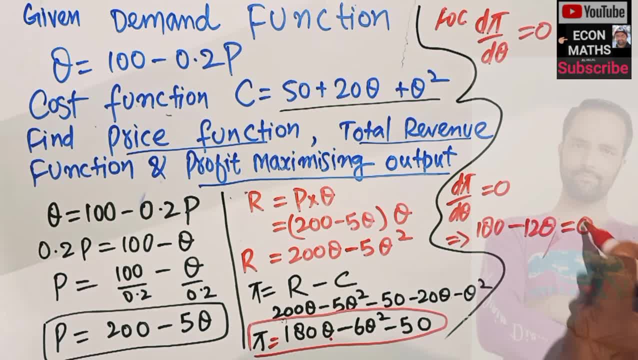 constant is 0.. So we are left with 180 minus derivative of Q. squared is 2Q, So 2, 6, 7, 12Q, So it will be equal to zero. Okay, So first order condition requires that marginal profit should.